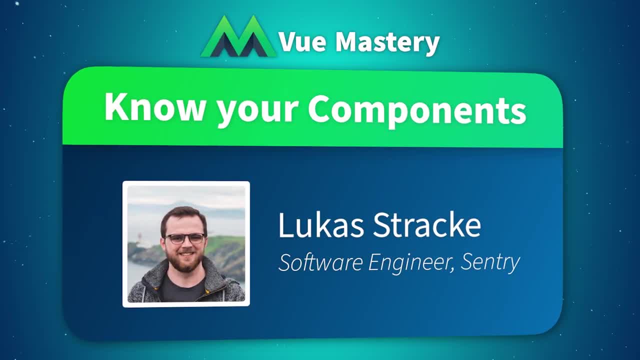 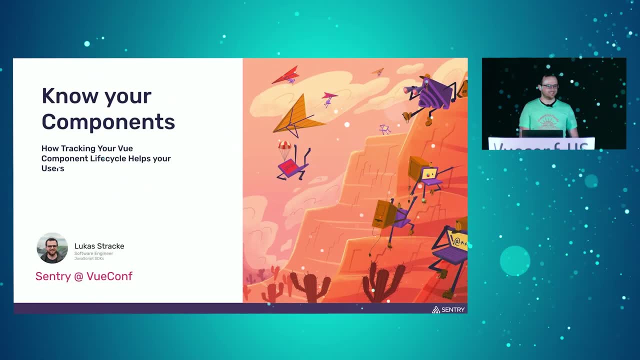 Hey everybody, it's great to be here. Great talk so far. So very quick. my name is Lucas and I work at Sentry. So, in a nutshell, Sentry captures errors that happen on your user's devices and it sends it basically to us and we tell you all about how this error happened, why it happened and where it occurred and stuff like that. 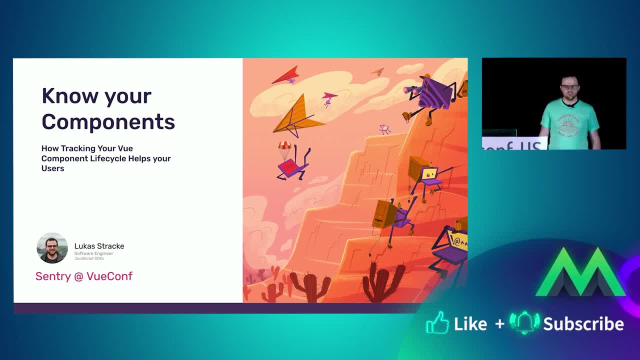 So, yeah, today, though I'm not really here to talk about Sentry or to pitch it, We can do this at the booth later on. Today I want to talk to you about view components and how tracking and analyzing our component lifecycle helps us basically get better insights into our performance of our apps and, yeah, overall, we'll make our users hopefully happier when we fix those performance problems. 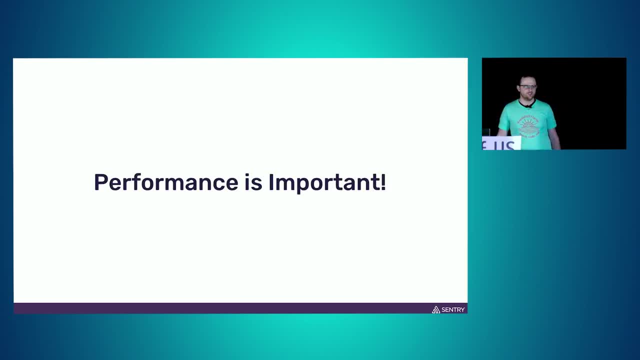 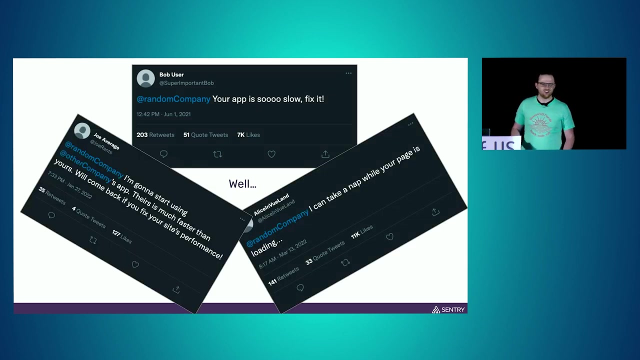 So let's get started with a fact which I think we hopefully can all agree on. We had a great talk about this. We had a great talk before on performance and view, So performance obviously is important, right? We want our apps to be snappy, to be quick, to be loaded quickly, and well, if our apps are not loaded quickly, well, we might get something like this, Or maybe something like this, Or maybe even something like this, And it might be on a subconscious level, but our users, they care about performance and if it's just not there, they're not going to be happy, right? So we don't want this to happen. 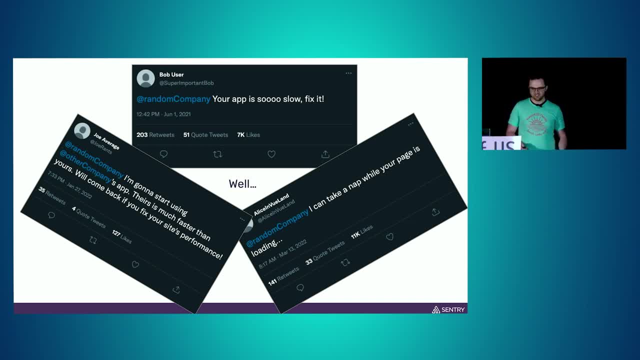 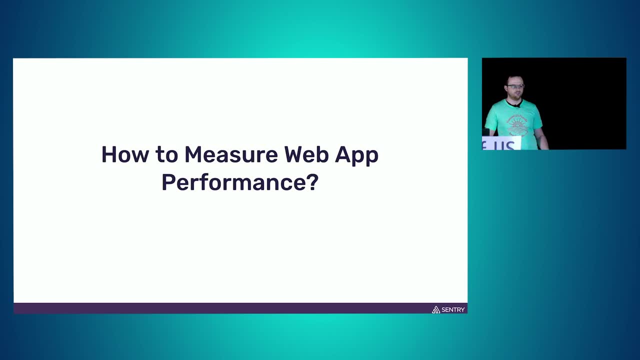 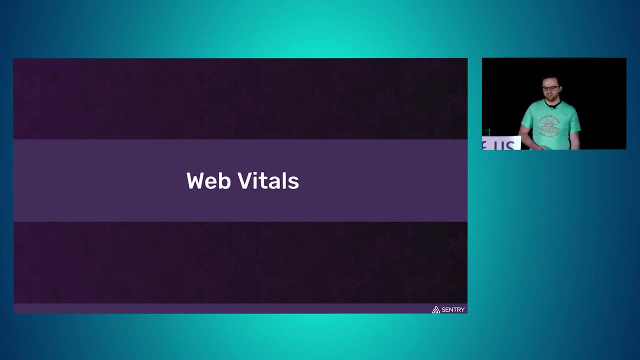 So well, What can we do about this? And the first thing that comes to our mind is, obviously we should kind of establish a baseline, right? We should measure how our apps currently perform. and well, how can we do this? So the good news is to get started on this. it's very simple. We've seen this before. We can basically just go into our dev tools in Chrome, to the performance tabs, and there we're going to see web vitals. 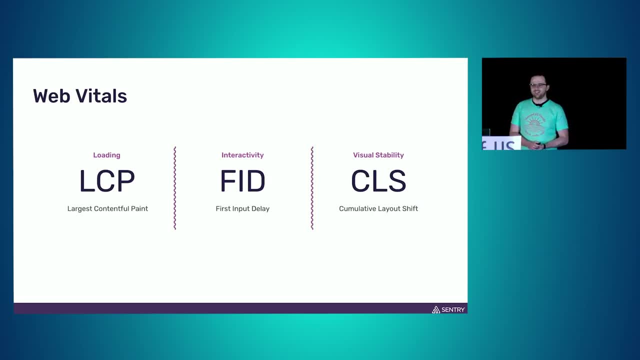 So web vitals, or again we've seen it before- they are basically a set of standardized metrics, right? We have some stuff for loading, we have some stuff for measuring interactivity and also for measuring visual stability or layout shift, right. 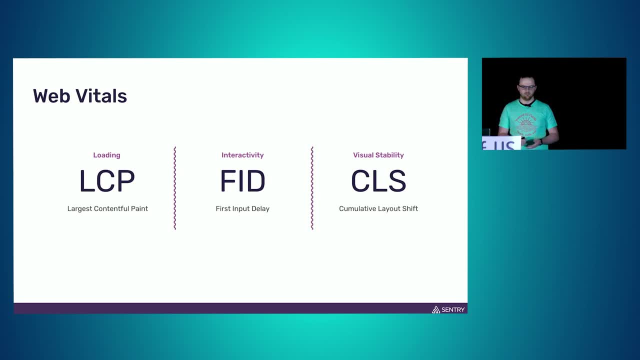 And they're great and they provide us a nice baseline of how our app is performing. But let's talk quickly about LCP for a second, because it shows us very well that there are certain limitations to web vitals. So many of those they're kind of based on heuristics, right? 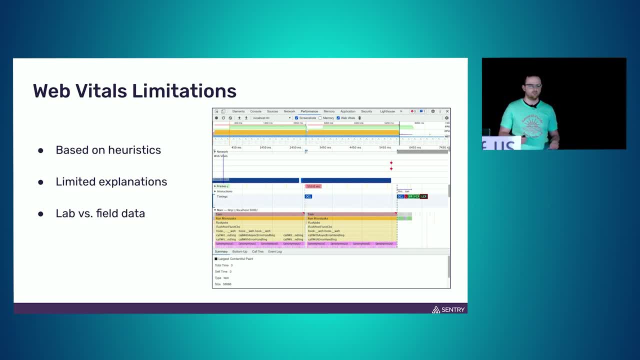 LCP, for example, we have to guess what is our biggest component or our biggest component Or our biggest element on the page, And maybe our browser gets this wrong. Maybe, for example, it takes our hero image or banner and kind of uses this. 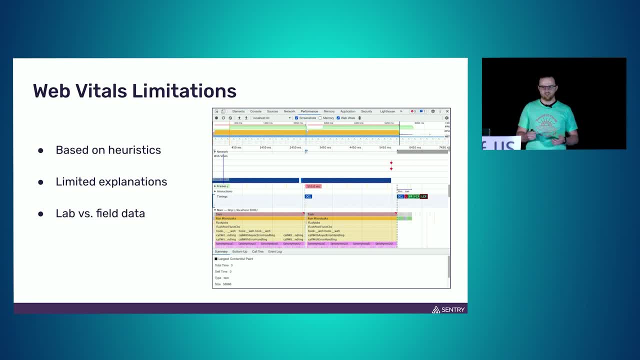 But what's actually much more important is, I don't know, the menu bar below it or some other text. So yeah, it's basically like heuristic, It can be wrong sometimes. Also, just LCP alone doesn't really provide us explanations as to why our page really got slow. 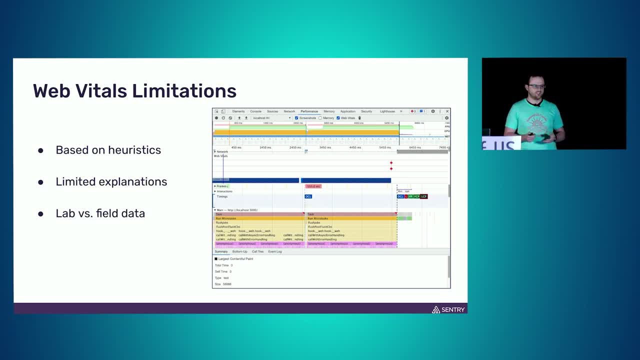 We have to dig deeper for that, And ultimately we have this discussion of lab versus field data. You know, when you're testing the stuff in your browser, when you build your app, you might get different results than when you're using it on your user's devices. 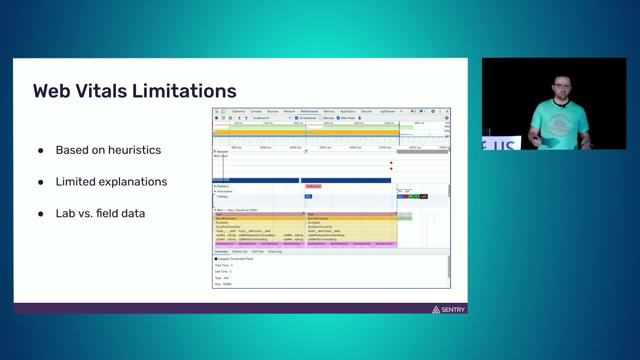 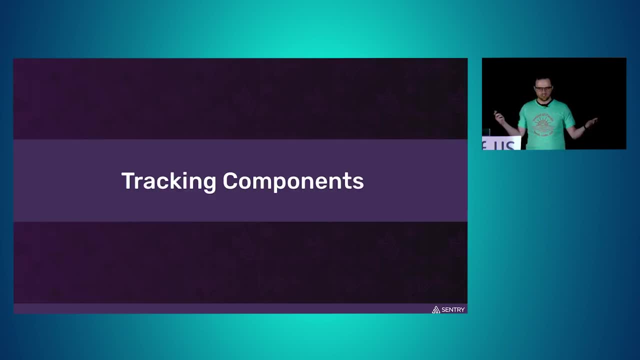 So, overall, it would be great to also get more information that comes directly from our user's devices. So well, how can we do better? Component tracking is the answer to that, And we can leverage this as developers because, well, we have components right. 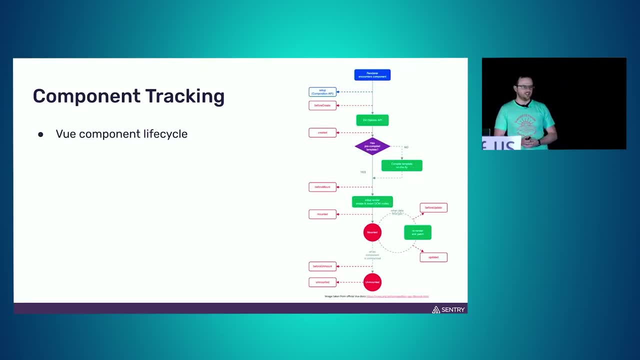 So what do I mean by that? I think we all know the new component lifecycle. You have these different stages that our component goes through- when it's initialized, when it's mounted, when it's updated or also then removed from the DOM- And we can leverage the hooks that are basically provided to us and just do some measurements. 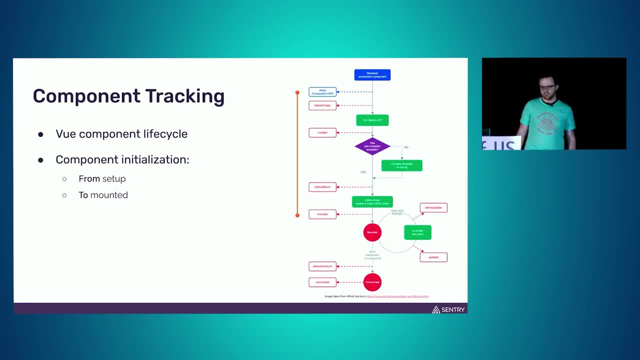 For example, we can measure the component initialization time, That is, from the setup phase, when our component is basically instantiated until it's mounted and therefore visible to the user in the DOM. So we can just measure the time and then we have basically component initialization time. 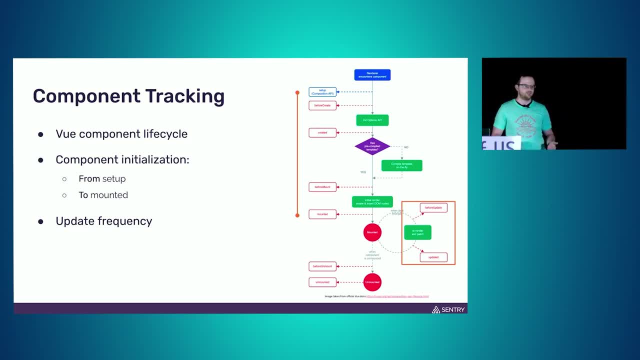 Or we can do some update measurements, like measuring update frequency or how long it takes to update stuff, And you know, for example, if your component gets updated a million times, then something might be wrong And we should kind of investigate that because this might imply a performance problem. 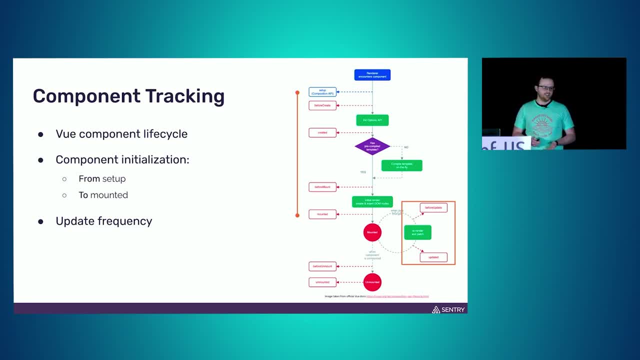 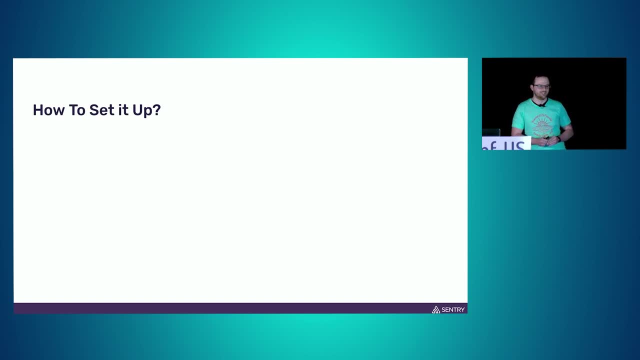 And yeah, so this is the idea basically. Now the question is: how can we do that? And the first step- and this is just kind of a half step to all of this- is basically just take a look at the browser DevTools again. 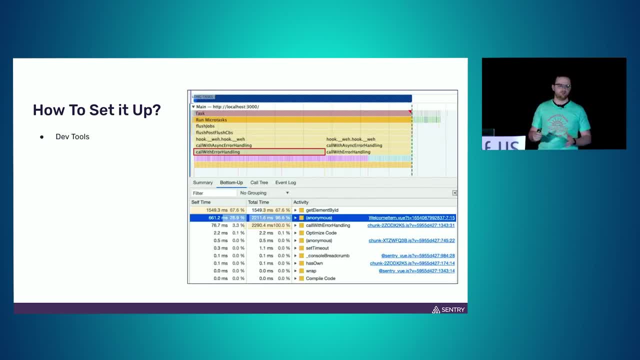 And there we can see these long-running tasks break down. And for example, here in this picture we see that our welcome item component for some reason took 600 milliseconds of continuous JavaScript evaluation time. And that's not great, because that obviously blocks our UI and people can't really use the app in the time. 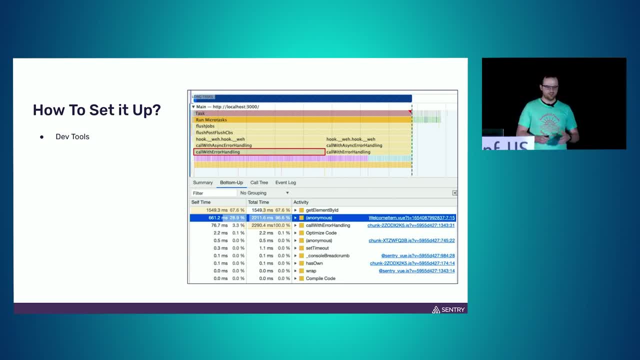 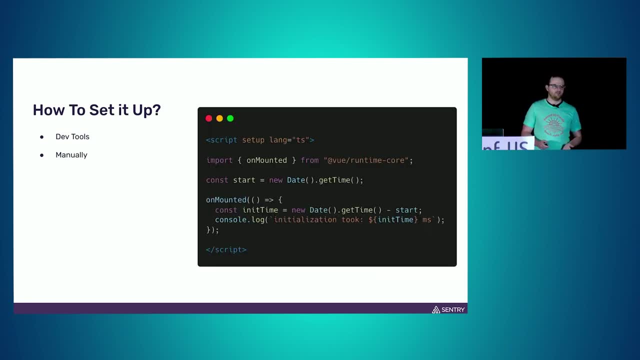 So we should definitely do something about this. So yeah, that's the first step, But it's not really easy. It doesn't scale really well, right? So next step: for that we have to kind of take our focus to our code. 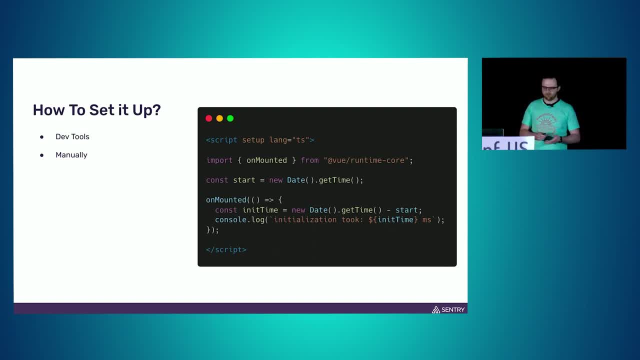 And we can kind of start doing it manually. We can just, for example, again measure component initialization time and then log it to the console, or better, send it to some server collect it right. But again this brings up the issue of scaling. 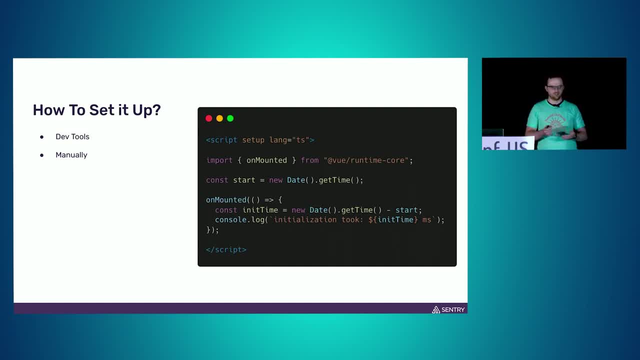 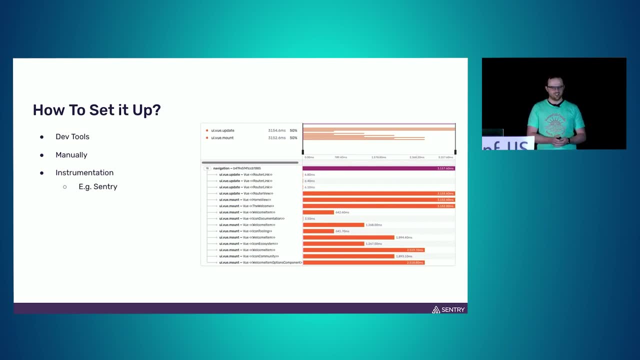 because if you have hundreds of components and multiple pages and whatever, this isn't really going to scale. well, So instrumentation is the answer to that. And well, surprise, surprise, Sentry does instrumentation. So what does it mean? Well, we actually hook into your components. 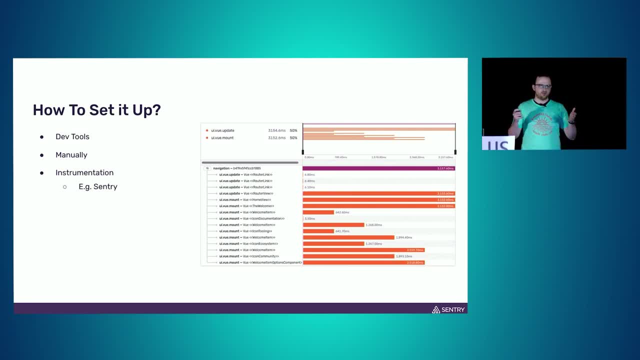 We do this via mixins And we do exactly like those measurements that I showed you before, Like, for example, measuring the mounting time until your component is visible, or updating time, And we collect this basically in something that we call spans. Those are the red things you can see here. 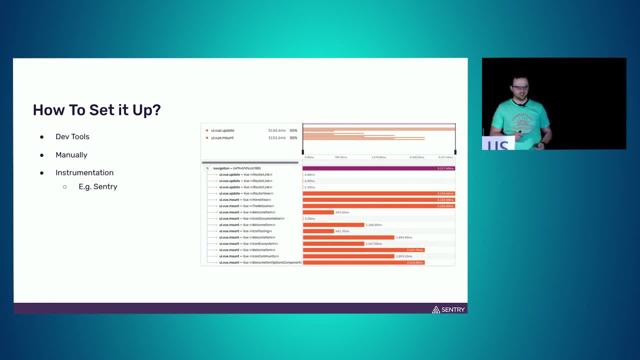 And we stack those on top of each other to get like what we call a transaction basically. And this gives us a lot of insight into the components and how, like, for example, one component- again this welcome component here. 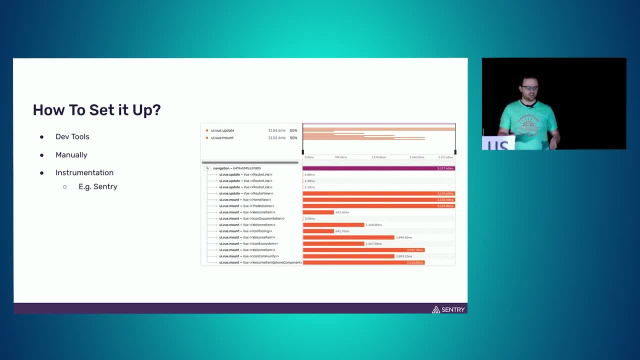 for example, influences the initialization time of all other components, And with that you can quickly drill down into your apps and just get to see which component is causing a slow page load, for example, or slow initialization time. So yeah, I'm not saying you have to use Sentry. 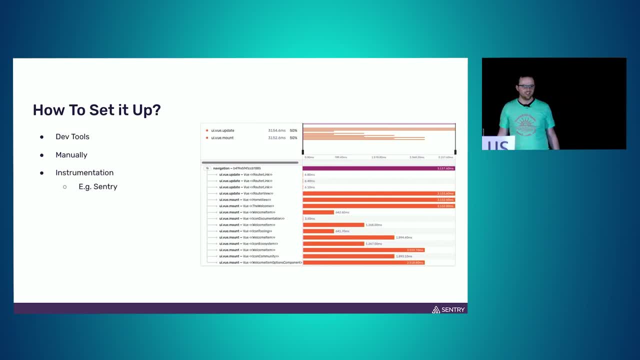 You can. of course, You can also just go into our GitHub. We're completely open source. Just copy our code. Copy what we're doing. Use any other tool. The main message here is: get to know your components and just start profiting from basically knowing what your components are doing. 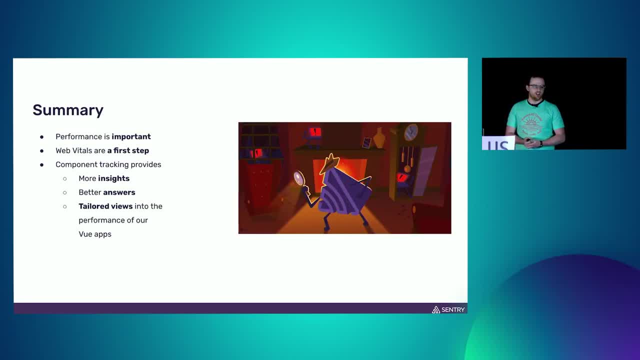 And yeah, with that, let's wrap this quickly up. Performance is important. We've seen this Web vitals. they're a great first step into, you know, getting the insets, And tools like Lighthouse also are really nice to have those audits. 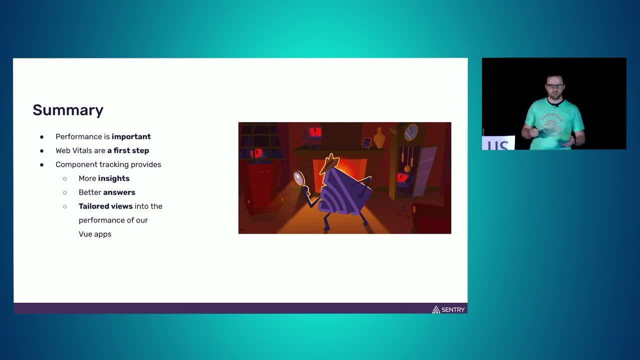 But if you want to go the extra mile and if you want to leverage what Vue gives us, which is components, then let's just track those components, Do it automatically. We get more insets, better answers and tailored views into the performance of our Vue apps. 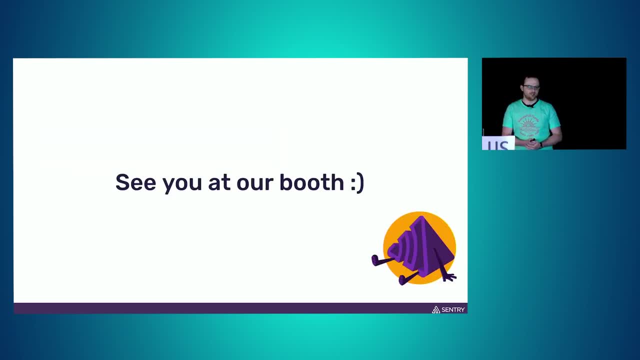 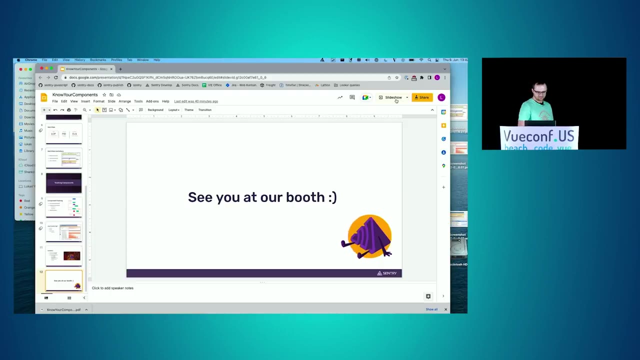 And yeah, that's basically it. Thank you very much for listening. If you want to talk about it a little more, see you at our booth. Happy to talk about it. And yeah, thanks for having me. We've got time for a couple quick questions. 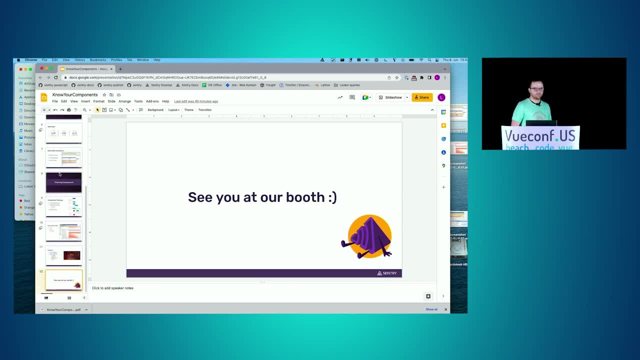 So if anybody has one for Lukas, please raise your hand. Anyone Anyone There, we go All right. Since you guys both raised your hand at the same time, you have to ask your question at the same time. So Do you guys have some sort of dashboard in which we collect this information and then 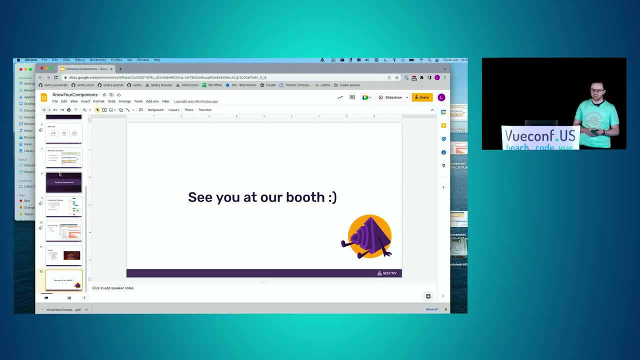 we can do further analysis. Yes, Great question. Yeah, We do have dashboards. We have a performance tab. So Central doesn't only do error monitoring, but also performance monitoring. So you can basically like Go in, start with your baseline and then do some improvements and you can see how you. 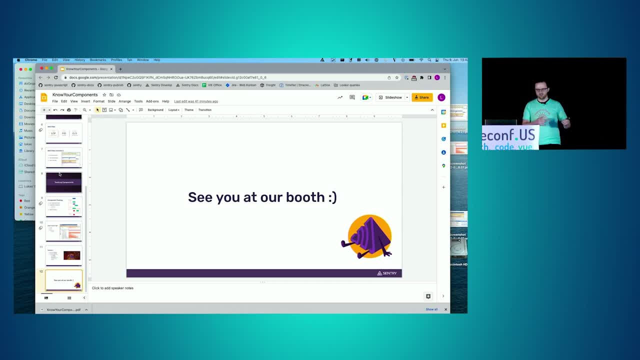 know your initialization time or also, like your web vitals, We do this as well- How these scores kind of evolve over time and get more insights on that, Hey, So obviously we want to do this in production to get useful data. 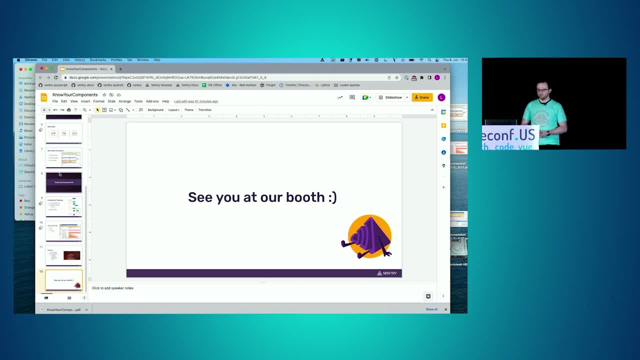 Yeah, So what's the overhead of hooking it to all the updates and tracing that and collecting the data? Well, I can answer that I can't lie right. There is going to be some overhead involved in this, but overall it depends really on. 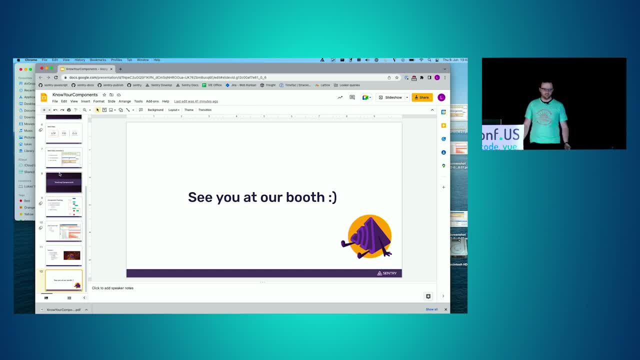 your application. Like, we try at Central to minimize this overhead as much as we can, but we have gotten some reports stating that, you know, when people basically instrument every single component on a page and there's like loads of components, then things are just going to get a little. 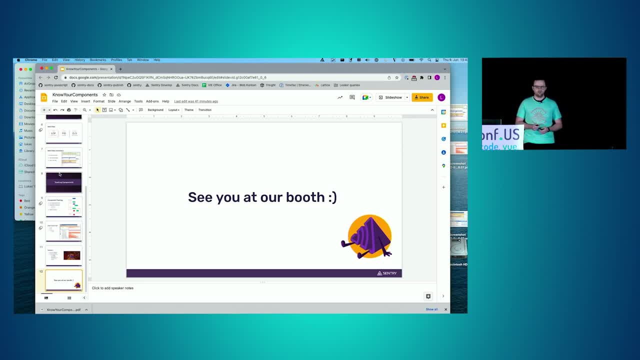 slower. So what we do is basically we kind of encourage our users to just instrument those components again that they think are important, And you can very well set this level of granularity basically in our settings. All right, Well, let's give it up for Lukas real quick.